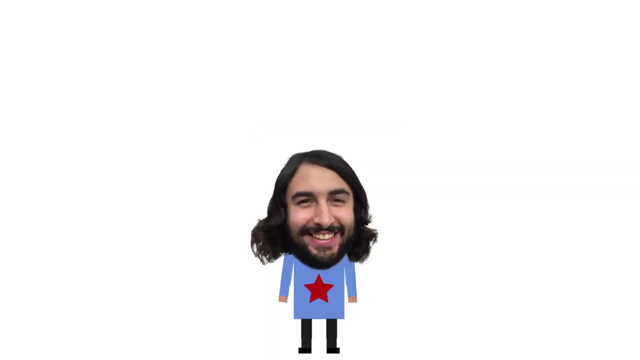 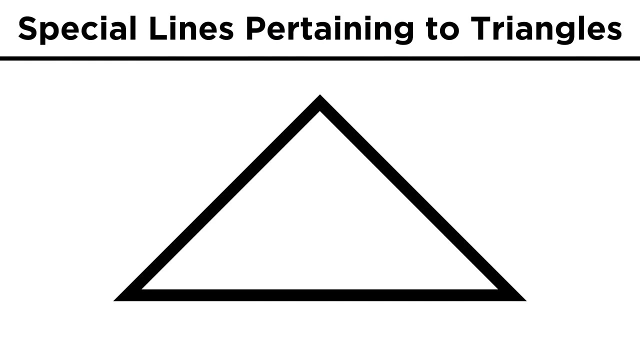 It's Professor Dave. let's learn more about triangles. Let's quickly identify some other lines that we can draw on triangles. One line we could draw is a perpendicular bisector. This is a line that is perpendicular to one of the sides of the triangle and cuts that. 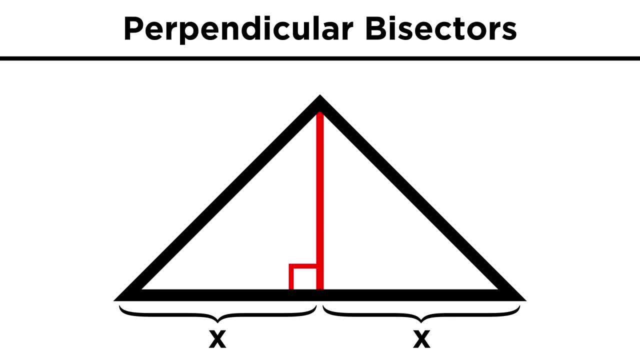 side into two line segments of equal length. Any point on this bisector must be equidistant from the endpoints of these line segments. so if the bisector also coincides with the other two sides, then these two sides must be equal and we have a right triangle. 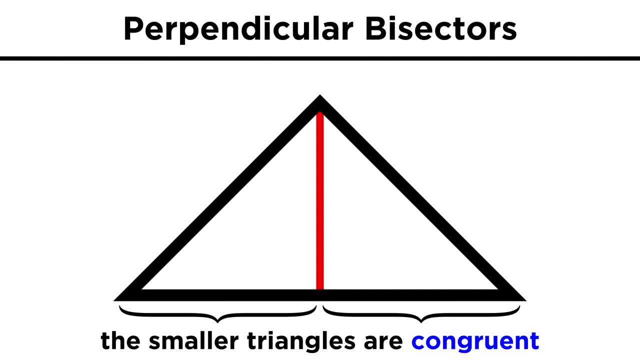 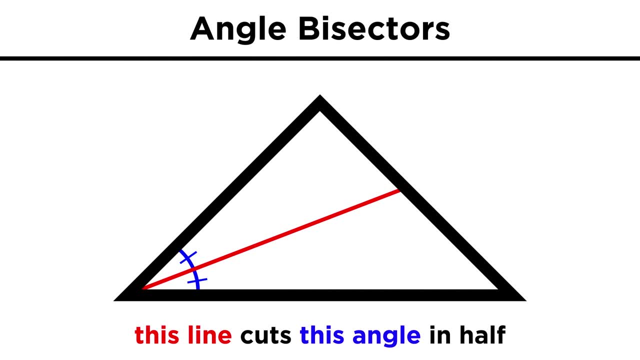 This also makes the two smaller triangles congruent. Besides perpendicular bisectors, we can also describe angle bisectors, which are lines that cut an angle in half. Any point on this angle bisector will be equidistant from the two other lines. 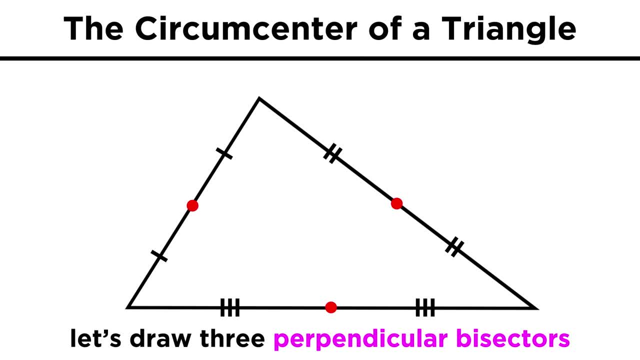 Now let's see what happens if we have a triangle and we try to draw three perpendicular bisectors, starting from the middle of each side. These extend from each midpoint at a ninety degree angle and meet at some location called the circumcenter of the triangle. 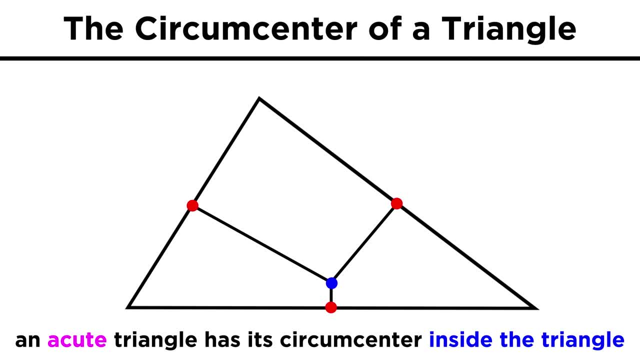 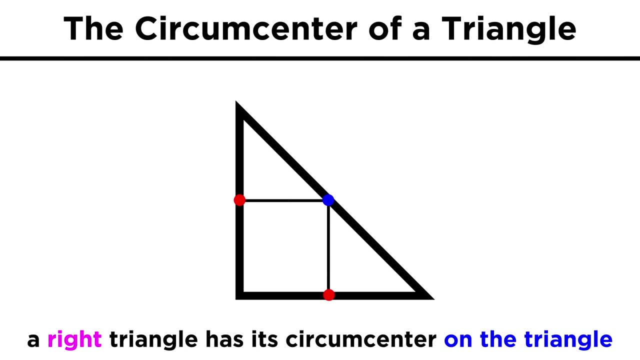 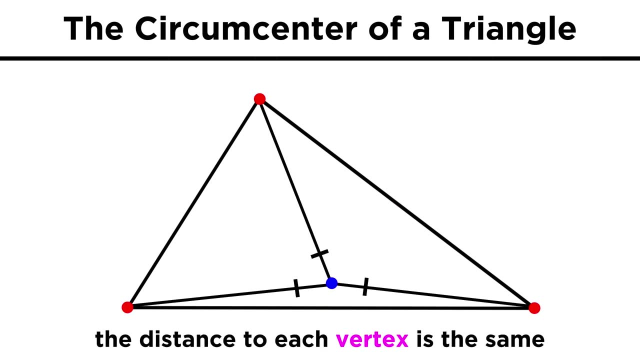 The circumcenter will be inside the triangle if it is acute, Outside of the triangle if it is obtuse, And on the triangle if it is a right triangle. While the distance to the sides of the triangle may differ, the circumcenter will be equidistant. 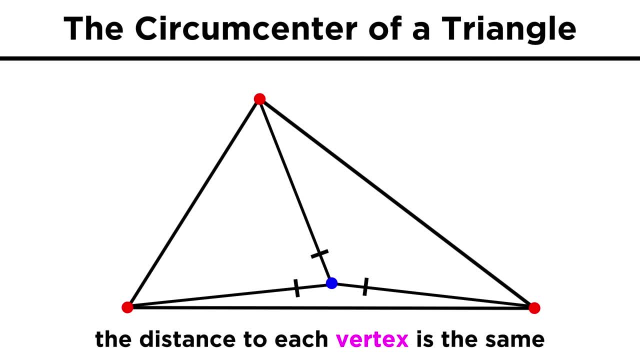 from the vertices of the triangle, meaning that the distance from the circumcenter to each corner is the same, no matter what type of triangle we are looking at. The circumcenter of the triangle will also be the center of the circle. The circumcenter of the triangle will also be the center of the circle. 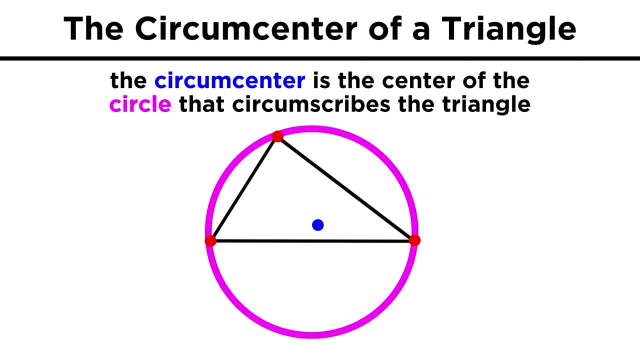 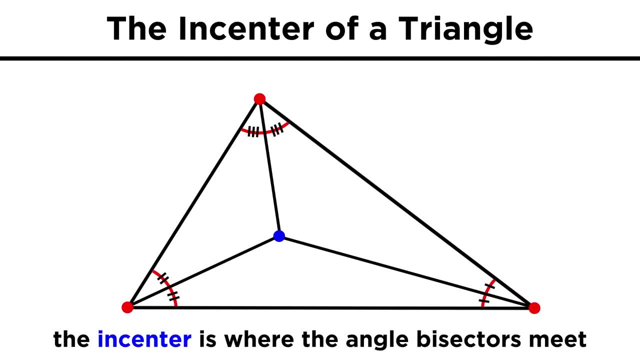 The circumcenter of the triangle will also be the center of the circle that circumscribes that triangle. This is the circle that contains all three vertices of the triangle. We can also discuss what happens if we bisect all the angles of a triangle. 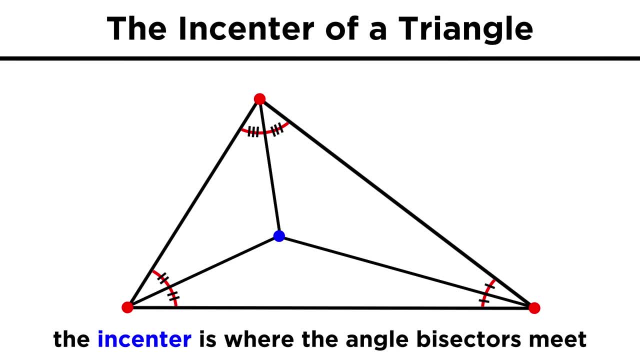 These angle bisectors will meet somewhere called the incenter of the triangle and, unlike the circumcenter, the incenter will always be inside the triangle. The incenter will be equidistant from the center of the triangle. The incenter will be equidistant from the sides of the triangle. so these three lengths. 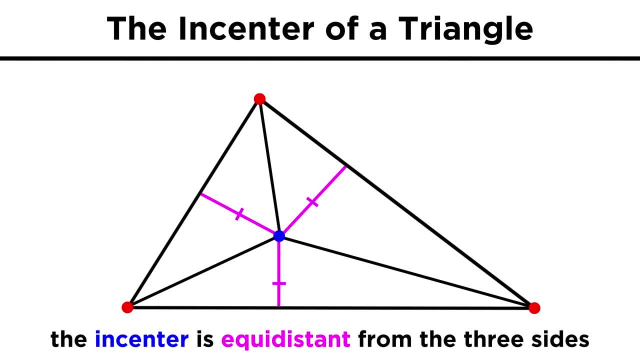 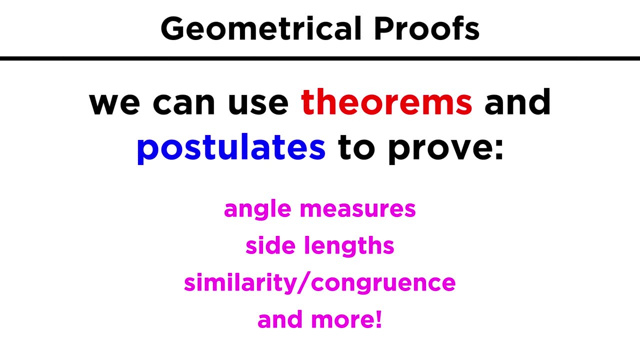 must be the same. The incenter will be the center of the circle that is inscribed in the triangle, which is the circle that intersects each side of the triangle at precisely one point. These theorems can be used to prove all kinds of things about various triangles, like the: 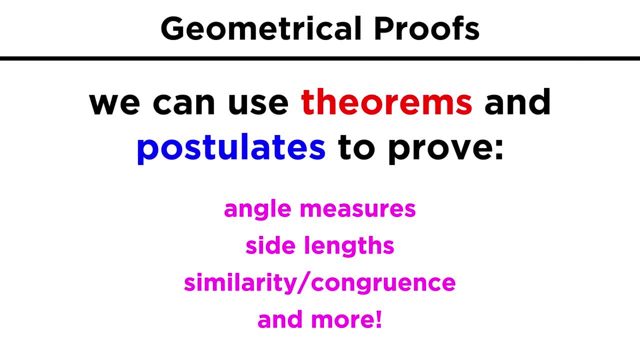 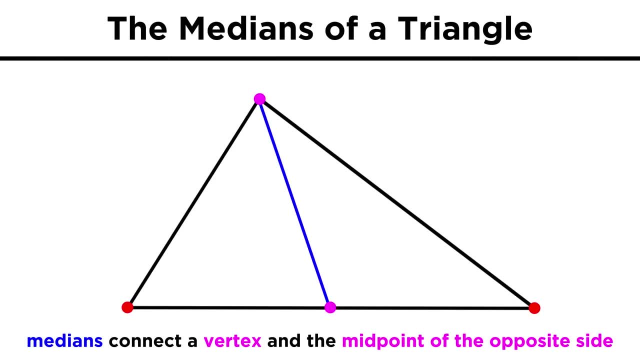 measures of certain angles and the lengths of certain line cetra and the lengths of certain linesets, segments. we just use the postulates strategically. Now, instead of a bisector, let's look at something called a median. A median of a triangle is a line segment that connects one vertex and the midpoint of the. 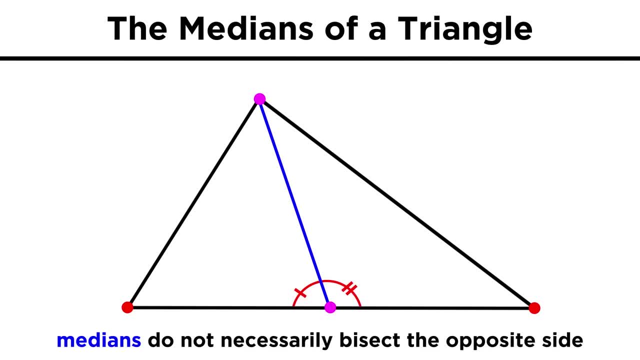 opposite side. Notice that this is not a bisector only because these are not right angles. If they were right angles, this median would also be a bisector and we would have a right angle. But it's not so. it's just a median. 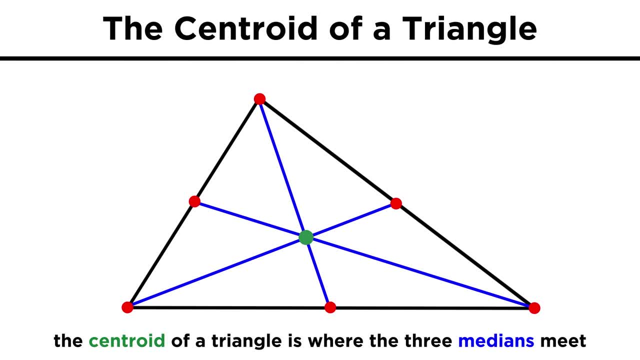 If we find the point where all three medians meet, this is called the centroid of the triangle and, like the incenter, this is always inside the triangle. The centroid is always two thirds of the way from one vertex to the opposite side, so that 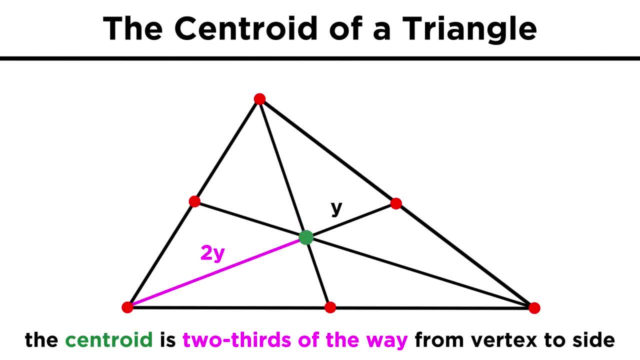 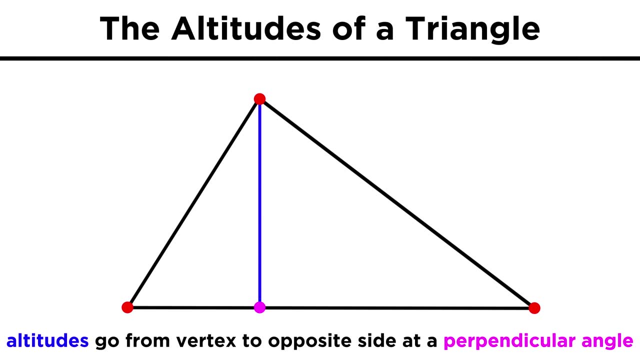 means that this distance is twice this, this distance is twice this and this distance is twice this. This allows us to determine the lengths of certain line segments given others. We can also identify the altitude of a triangle. This is what we get when we start from a vertex and make a line segment that extends towards. 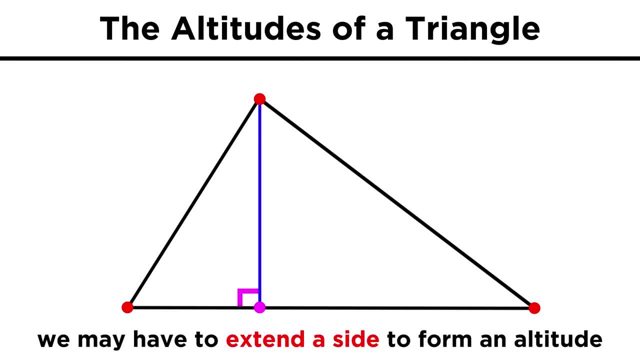 the opposite side in perpendicular fashion. If we have to extend the opposite side in one direction or the other to get this, that's what we do. We just need to make a right angle. Each triangle has three altitudes. Each triangle has three angles.